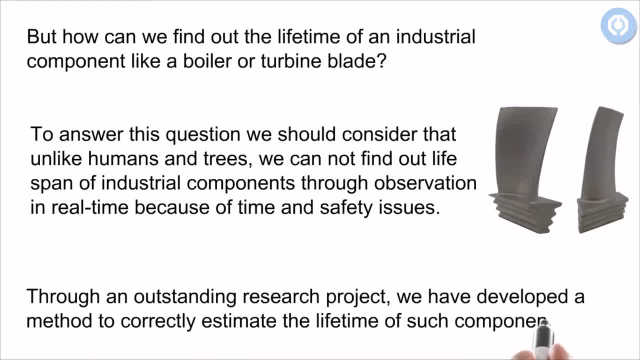 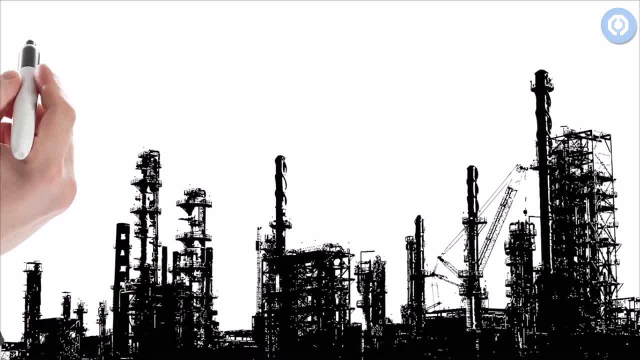 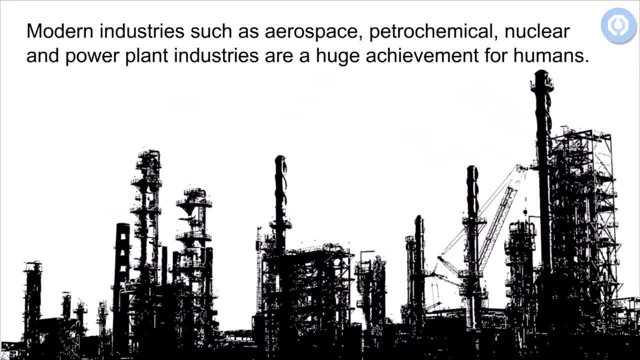 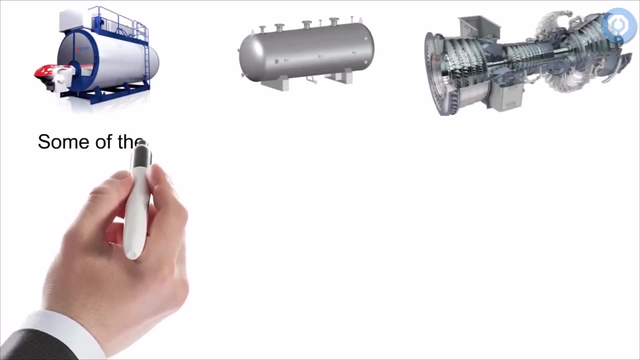 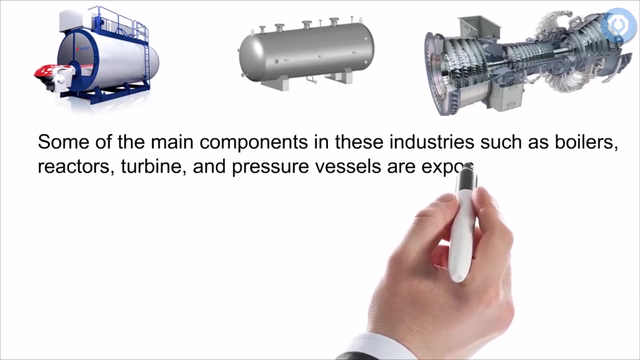 Modern industries such as aerospace, petrochemical, nuclear and power plant industries are a huge achievement for humans. Some of the main components in these industries, such as boilers, reactors, turbine and pressure vessels, are exposed to loading conditions that involve long-term high temperature and forces. 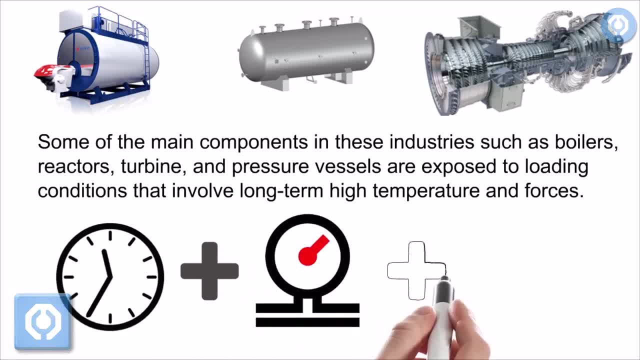 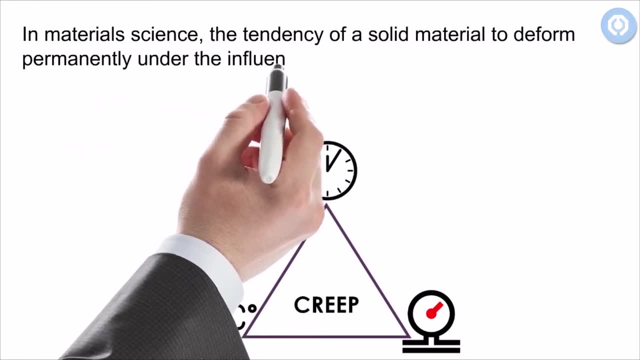 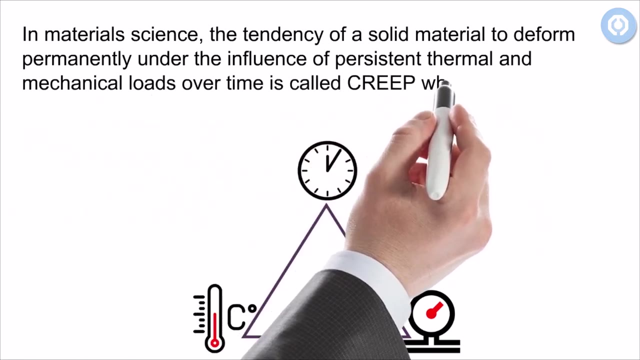 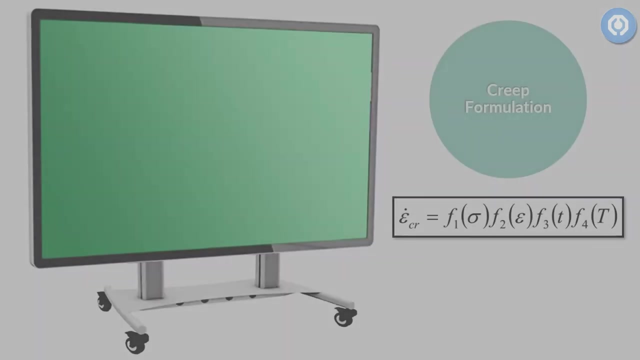 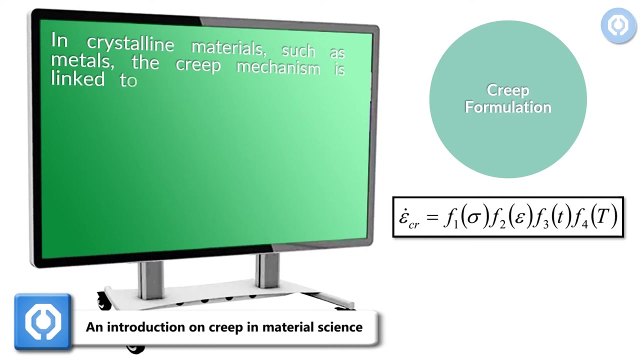 In materials science, the tendency of a solid material to deform permanently under the influence of persistent thermal and mechanical loads over time is called creep, which is an irreversible process. In crystalline materials such as metals, the creep mechanism is linked to the diffusional 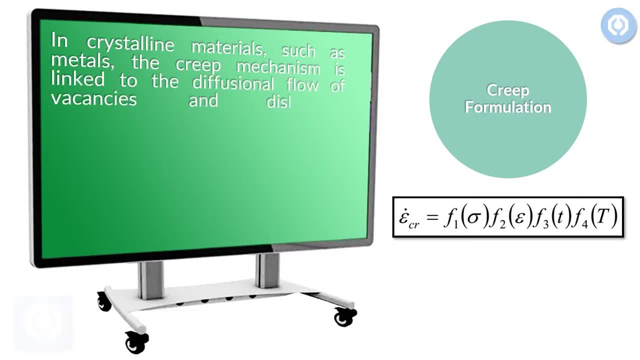 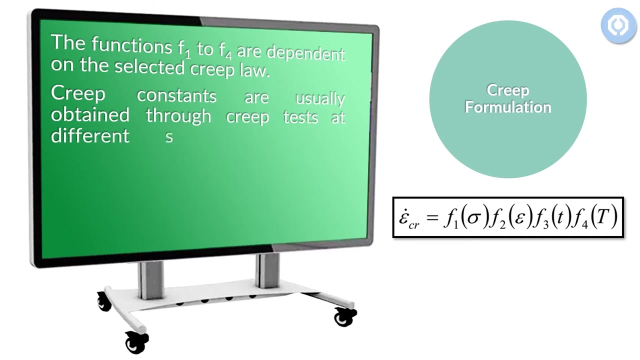 flow of vacancies and dislocation movement. The dependency of creep deformation on stress, strain, time and temperature are generally modeled as the shown formula. The functions F1 to F4, are dependent on the selected creep law. Creep constants are usually obtained through creep tests at different stress levels and 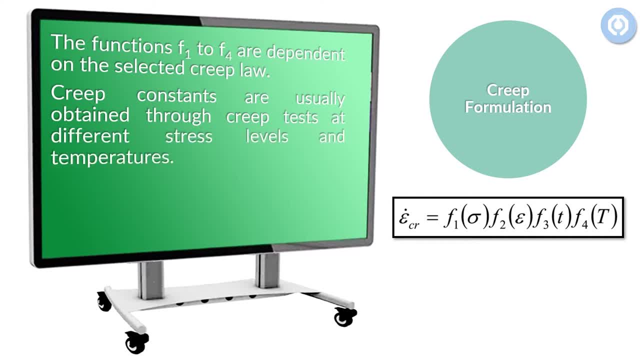 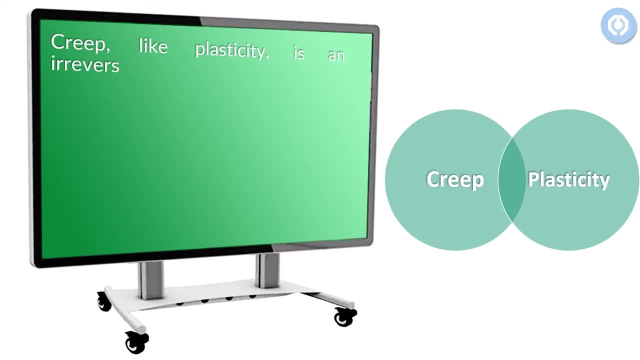 temperatures. Creep, like plasticity, is an irreversible strain and the material is a solid material, It is assumed to be incompressible. On the other hand, creep, unlike rate-independent plasticity, has no yield surface at which plastic-saint rains occur, and creep-saint rains are assumed to develop at all non-zero. 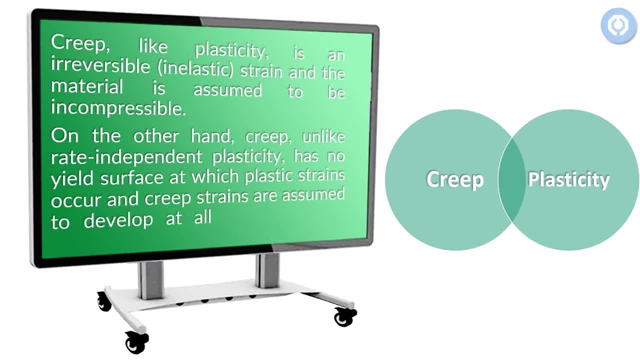 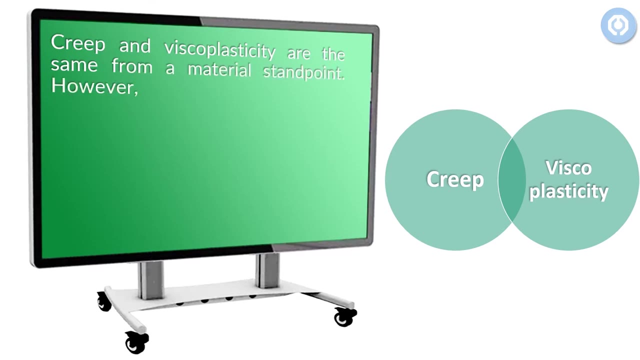 stress values. Creep and viscoplasticity are the same from a material standpoint. Creep and viscoplasticity are the same from a material standpoint. However, creep is generally used to describe a thermally activated process with a low strain rate. 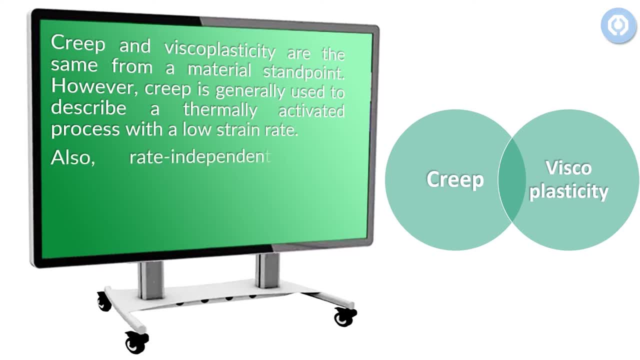 Also rate-independent. plastic saint rains and creep saint rains are treated in a weakly coupled manner. Conversely, viscoplasticity models are used to describe high strain rate applications, for example, impact loading and inelastic saint rains are treated in a strongly coupled manner. 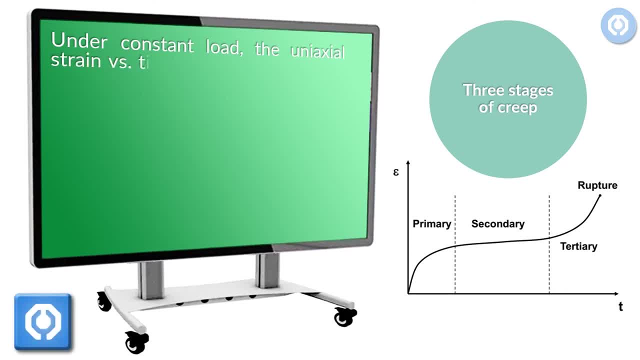 Under constant load. the uniaxial strain versus time behavior of creep is shown in the following figure. In the primary stage, the strain rate decreases with time. This trend occurs over a short period. The secondary stage has a constant strain rate. In the tertiary stage, the strain rate increases rapidly until failure. 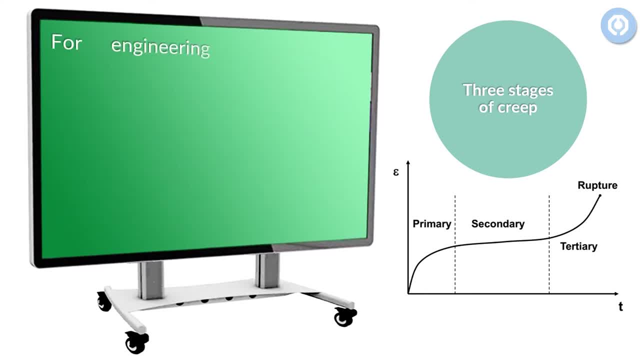 For engineering analysis, the primary and secondary stages of creep are usually of greatest interest. Tertiary creep is usually associated with the onset of failure and is short-lived. The strain rate in primary creep is usually greater than the strain rate in tertiary creep. However, the strain rate is decreasing in the primary stage, whereas it is usually nearly constant in the secondary stage. 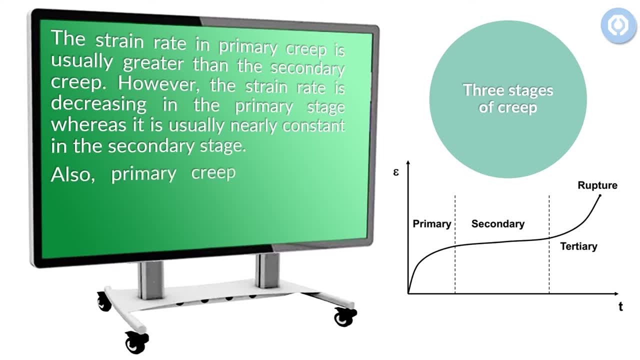 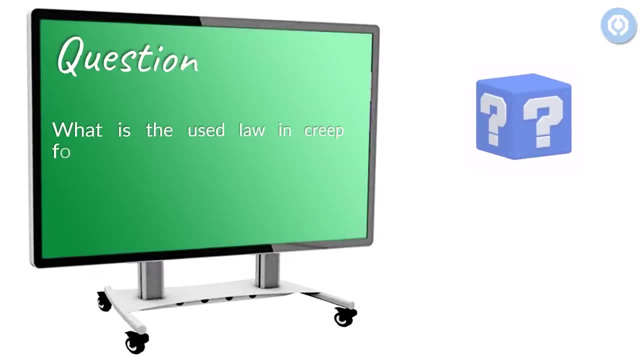 Also, primary creep occurs in a shorter time period than secondary creep. Question: What is the used law in creep formulation for temperature dependency? The answer is that the strain rate increases with time and when the strain rate decreases with time, the creep process decreases. 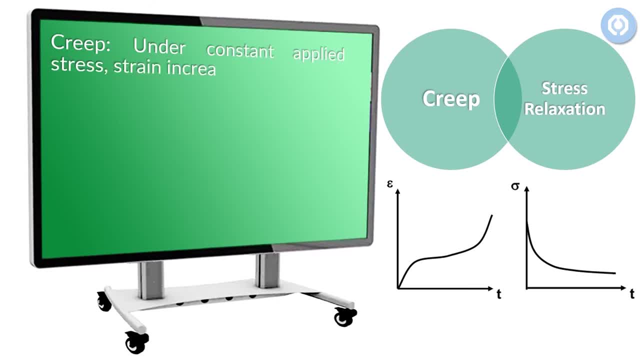 When under constant applied stress, strain increases, we have a creep process and when, under constant applied strain, stress decreases, we have a stress relaxation process. Time hardening assumes that the creep strain rate depends only upon the time from the beginning of the creep process. 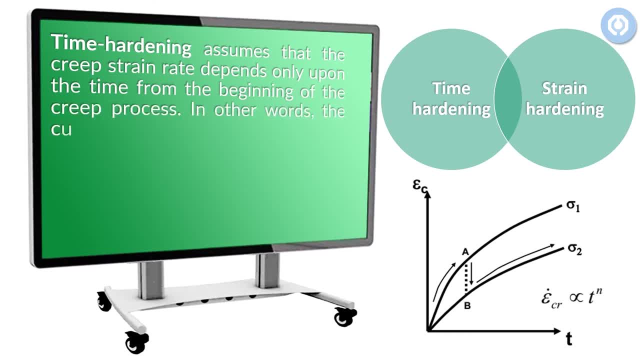 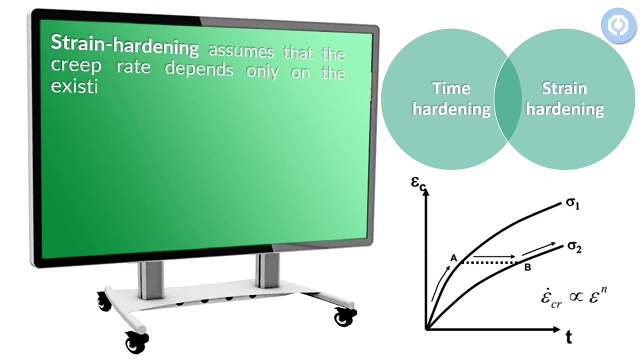 In other words, the curve shifts up and down As stress changes from sigma 1 to sigma 2, the different creep rates are calculated at points A to B. Strain hardening assumes that the creep rate depends only on the existing strain of the material. 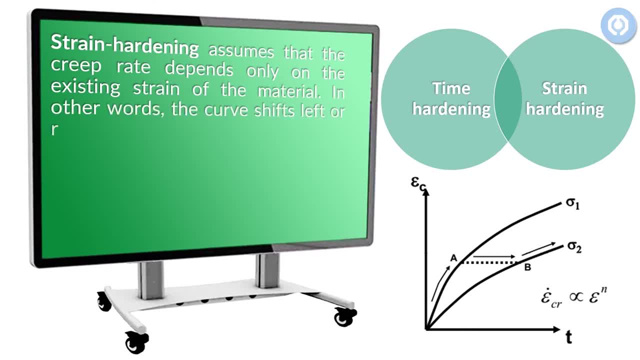 In other words, the curve shifts left and right As stress changes from sigma 1 to sigma 2, the different creep strain rates are calculated at points A to B. Strain hardening assumes that the creep strain rate depends only upon the existing strain of the material. 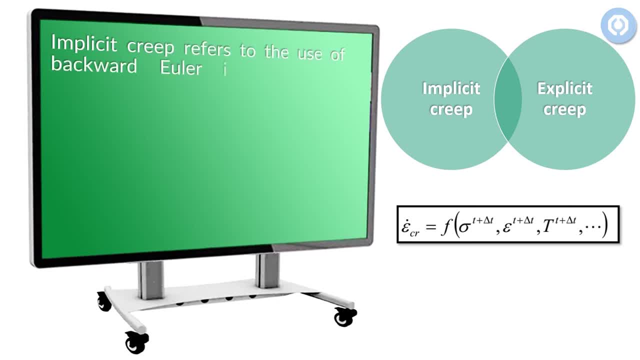 Implicit creep refers to the use of backward Euler integration for creep-Saint-Rheims. This method is enumerically unconditionally stable. This method is enumerically unconditionally stable. This method is numerically unconditionally stable reigns that it does not require a smaller time step as the explicit creep method, so it is much faster. 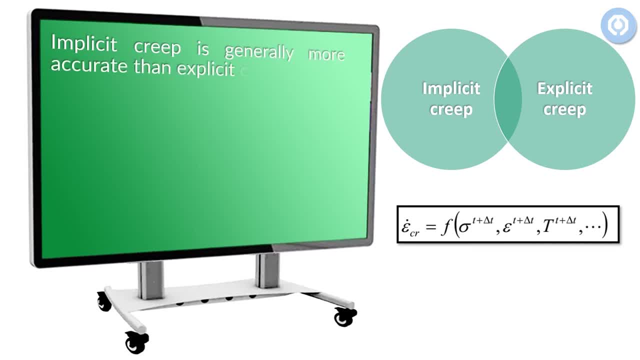 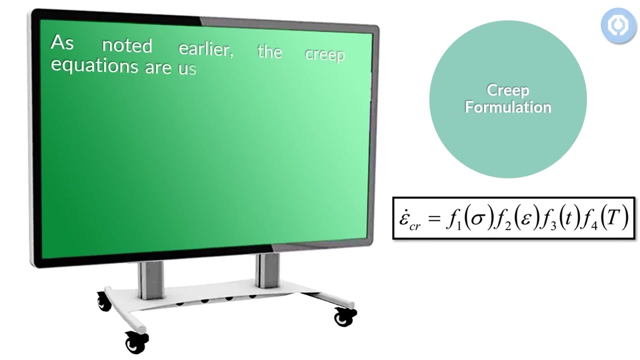 Implicit creep is generally more accurate than explicit creep, but it is still dependent on the time step size. A small enough time step must be used to capture the path-dependent behavior accurately. As noted earlier, the creep equations are usually of a rate form similar to the shown. 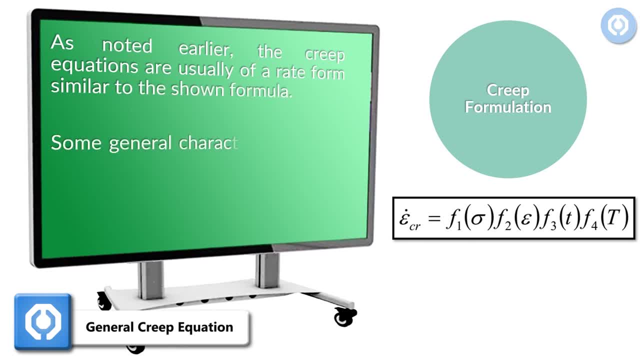 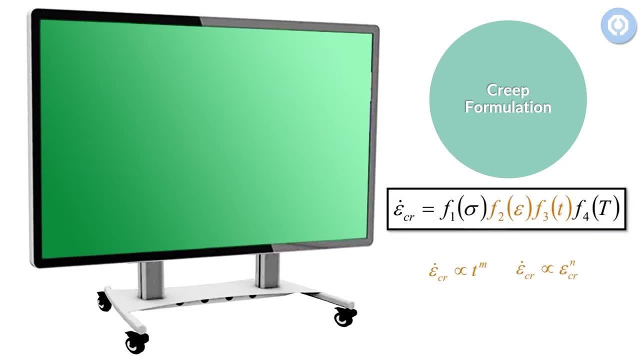 formula. Some general characteristics will be discussed here. Primary creep usually exhibits either time or strain hardness. Time-hardening formulation is the inclusion of a time-dependent term and strain-hardening formulation is the inclusion of a strain-dependent term. Secondary creep does not exhibit time or 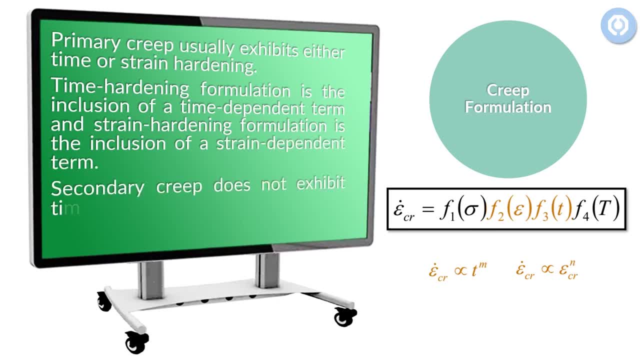 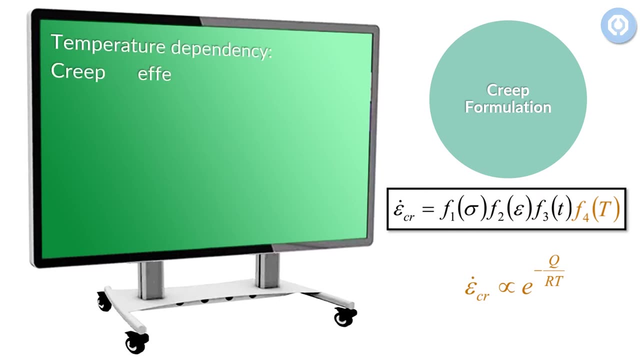 strain-hardening and creep strain rate is usually constant. Temperature dependency: Creep effects are thermally activated and its temperature dependence is usually expressed through the Arrhenius law, Where Q is the activation energy, R is the universal gas constant and T is the absolute temperature. 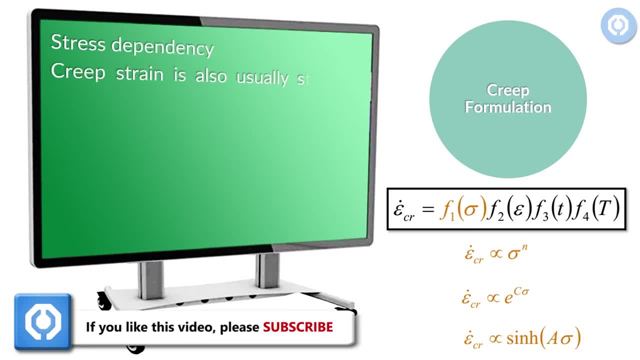 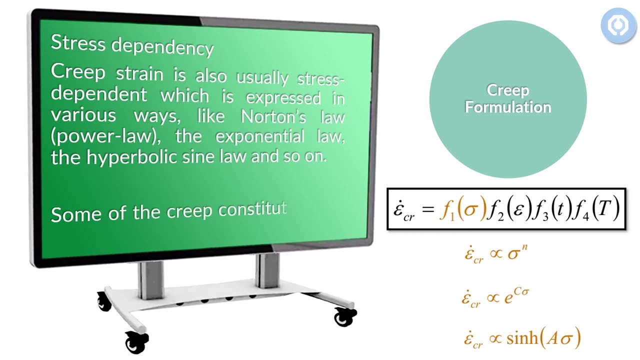 Stress dependency. Creep strain is also usually stress-dependent, which is expressed in the various ways like Norton's law or power law, the exponential law, the hyperbolic sinus law and so on. Some of the creep constitutive laws are presented here. 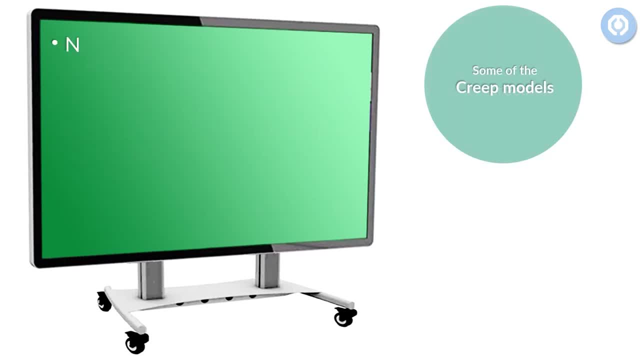 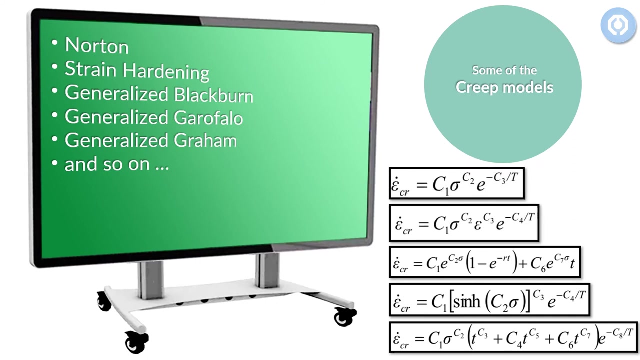 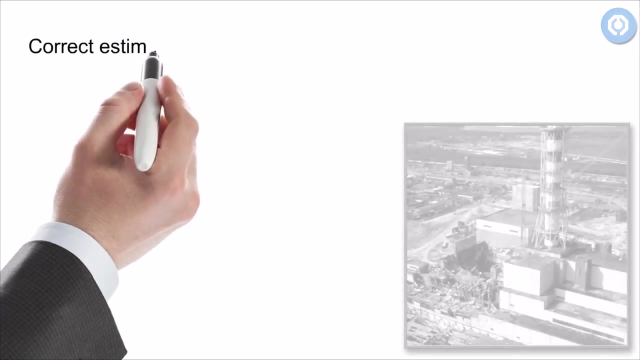 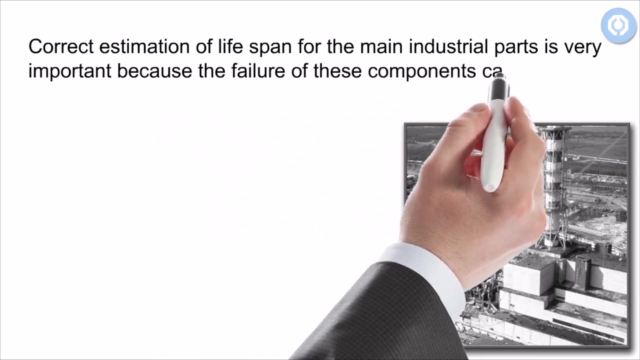 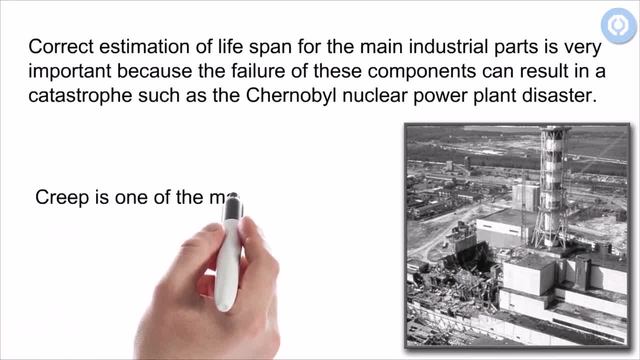 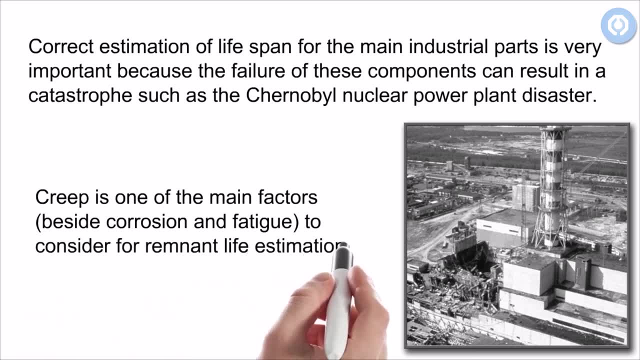 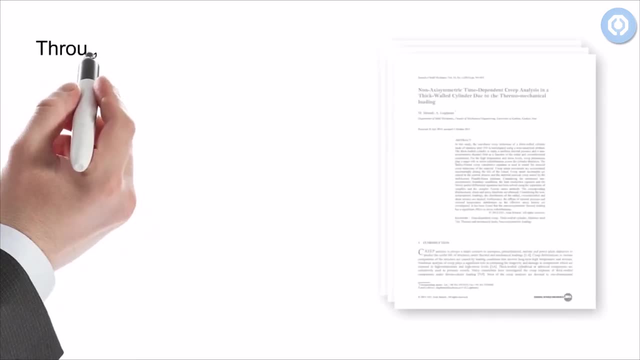 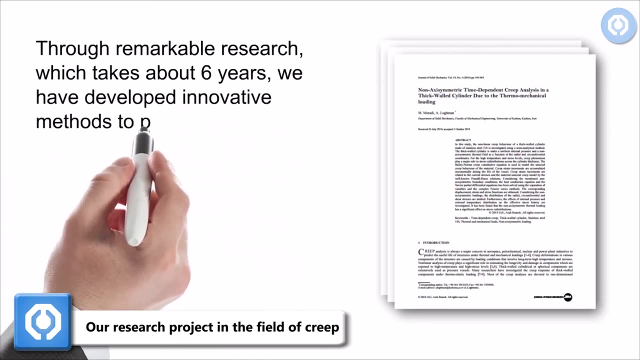 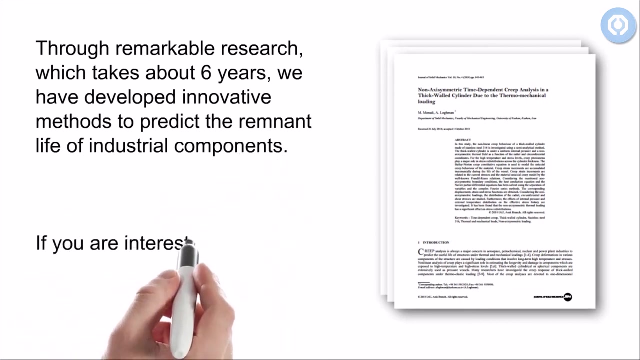 The compulsory narcissist is a price of même bewusst fatigue to consider for remnant life estimation of components. Through remarkable research which takes about six years, we have developed innovative methods to predict the remnant life of industrial components. If you are interested in this subject, find more specific information through our published